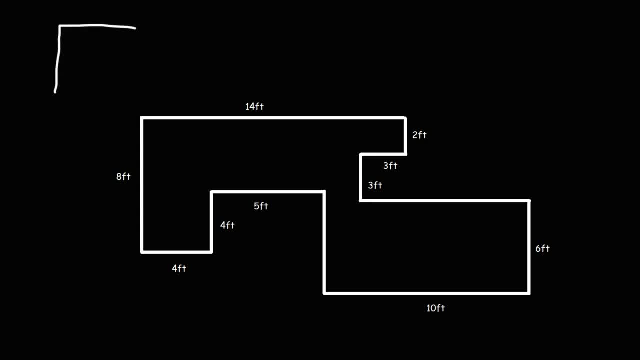 So let's say we have- let me draw a better rectangle. Let's say we have a rectangle and we know the length and the width of the rectangle. So let's say the width of the rectangle is 4 feet and the length of the rectangle is 5 feet. 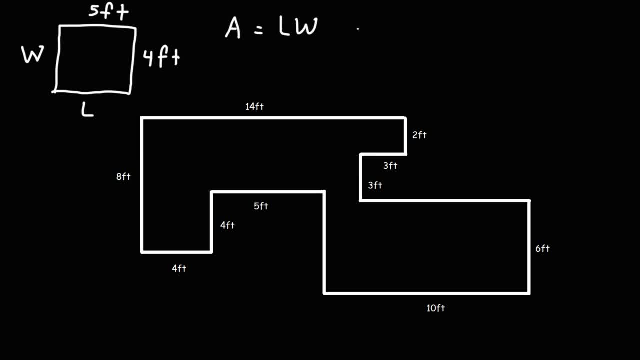 The area is going to be length times width, So it's 5 feet times 4 feet. 5 times 4 is 20, and feet times feet is square feet. So when dealing with area, you're always dealing with square units such as square feet, square inches. 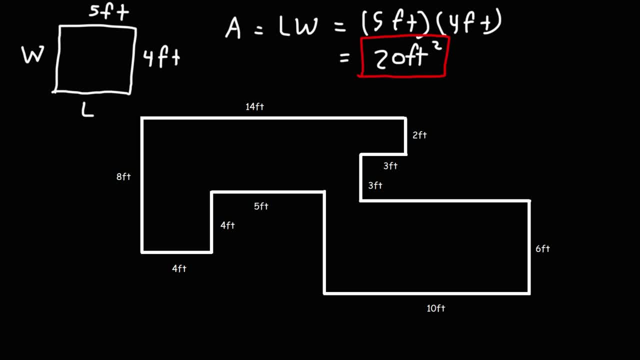 Square yards, square meters. When dealing with volume, you're dealing with cubic feet, cubic meters, cubic inches and so forth. So that's how we can calculate the square footage of a rectangular area. So what we're going to do in that problem, or in this problem, rather, 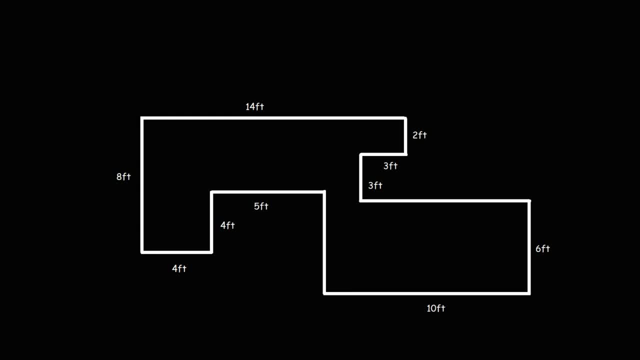 is, we're going to break up this composite figure into smaller sections, smaller rectangles. We're going to calculate the area of each rectangle and then find the sum. So let's Start with this rectangle. We can see that it's 4 by 4.. 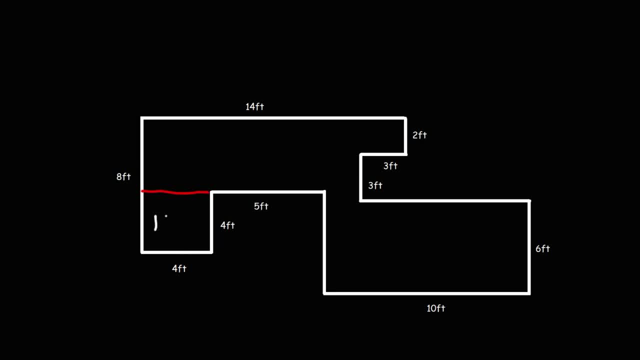 So 4 feet times 4 feet gives us an area of 16 square feet. Now let's calculate the area of this rectangle. So this is 10 feet by 6 feet. 10 times 6 will give us an area of 60 square feet. 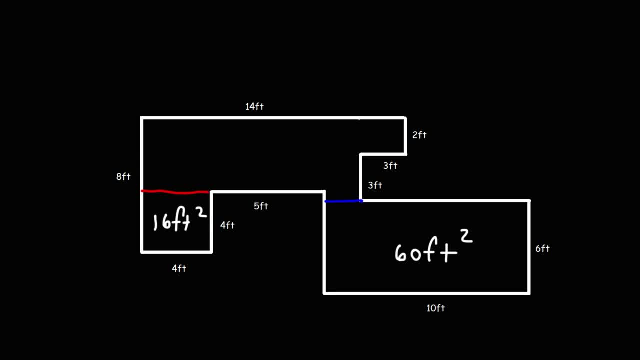 Now let's calculate the area of the rectangle on the upper right, So it's 2 by 3, which will give us an area of 6 square feet. Now, what else can we do? I recommend drawing a line here. So let's get the area of this region on the upper left. 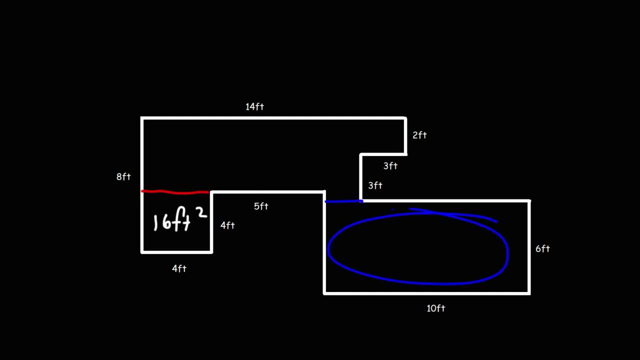 Now let's calculate the area of this rectangle, So this is 10 feet by 6 feet. 10 times 6 will give us an area of 60 square feet feet. Now let's calculate the area of the rectangle on the upper right, So it's 2. 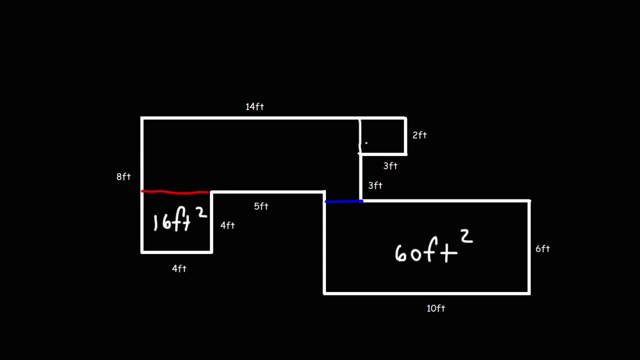 by 3, which will give us an area of 6 square feet. Now, what else can we do? I recommend drawing a line here, So let's get the area of this region on the upper left. So first I'm going to redraw the figure. Note that the length is not 14. 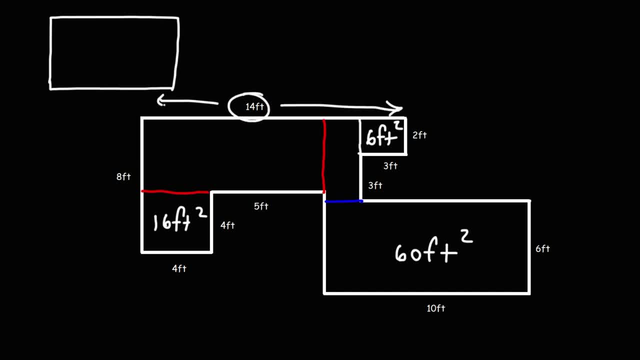 feet. 14 feet spans this entire distance. Rather, the length of that rectangle is the sum of these two. 4 plus 5 will give us the rectangle of this area, which is 9.. I mean the length of that area which. 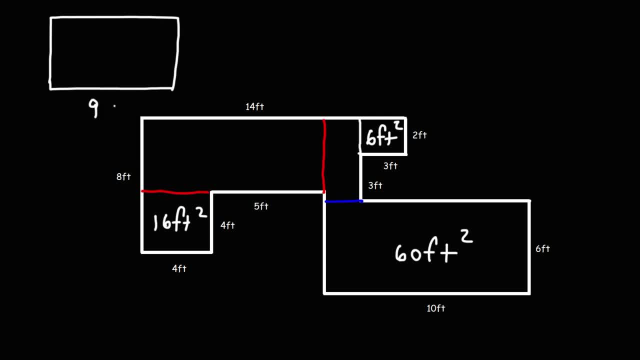 is 9 feet. Now the next thing that we need is the width of this section. Now, this entire distance spans 8 feet and this portion here is 4 feet. So the difference between 8 and 4 will give us the width of the rectangle under. 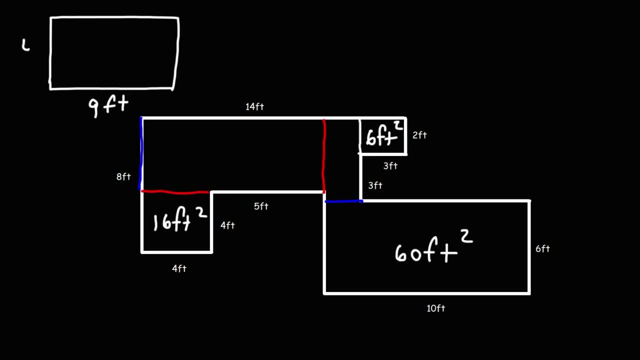 consideration, and that's going to be 4 feet. So 4 times 9 gives us an area of 36 square feet. So now let's get rid of that and let's calculate the area of the final piece. So I'm going to redraw. 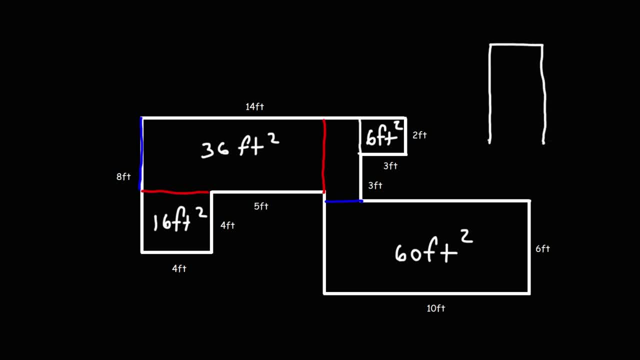 that figure here. So we're focused on this section. So the width is going to be 2 plus 3.. If we add these two, we get a width of 5 feet. Now we need to determine the length, which is this section here. 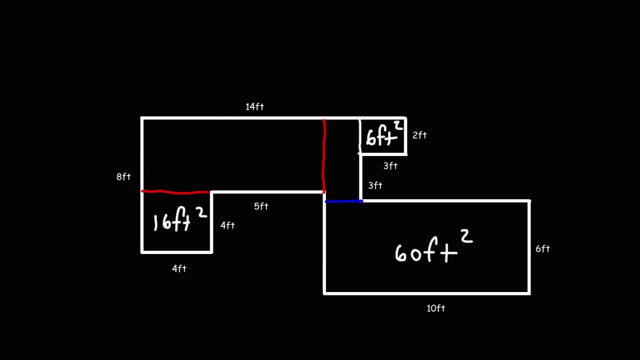 So first I'm going to redraw the figure. Note that the length is not 14 feet. 14 feet spans this entire distance. Rather, the length of that rectangle is the sum of these two. 4 plus 5 will give us the rectangle of this area, which is 9.. 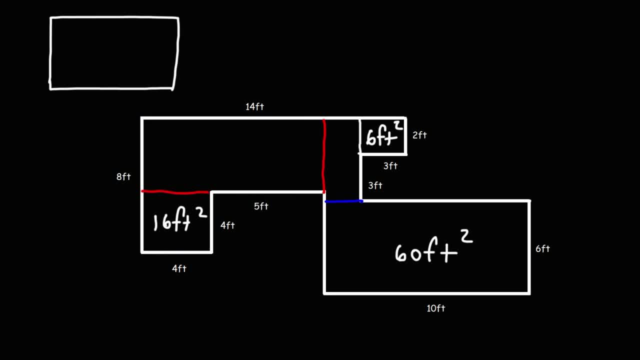 I mean the length of that area, which is 9 feet. Now, the next thing that we need is the width of this section. Now, this entire distance spans 8 feet And this portion here is 4 feet. So the difference between 8 and 4 will give us the width of the rectangle under consideration. 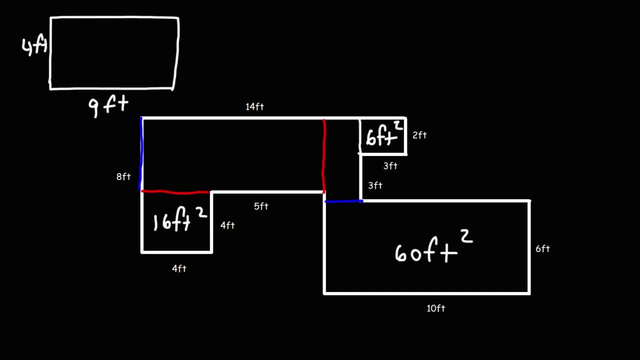 And that's going to be 4 feet. So 4 by 4 is 8 feet. So 4 by 4 is 8 feet. So 4 times 9 gives us an area of 36 square feet. So now let's get rid of that. 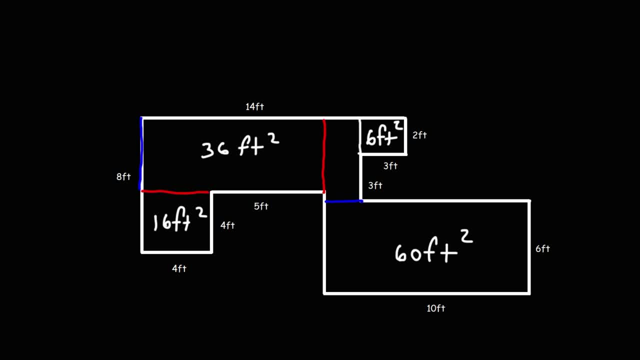 And let's calculate the area of the final piece. So I'm going to redraw that figure here, So we're focused on this section. So the width is going to be 2. Plus 3. If we add these two we get a width of 5 feet. 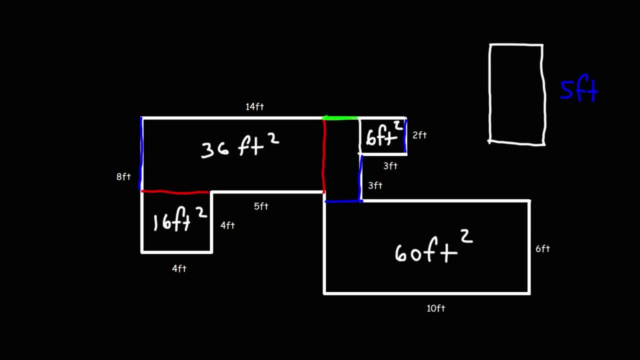 Now we need to determine the length, which is this section here. How can we do that? Well, we know this entire distance is 14 feet, And if we add these two, 4 plus 5.. We know that this section 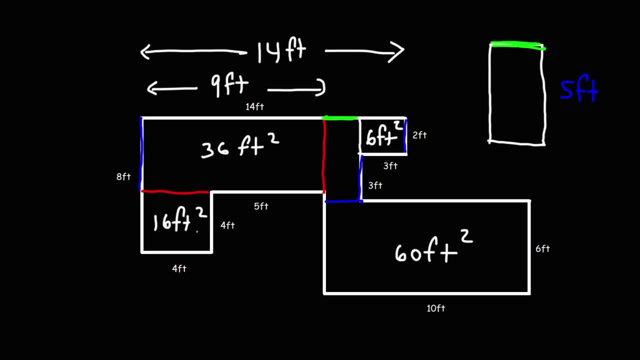 Is 9 feet And looking at this piece here, this is 3 feet long. So to get the, The length of the rectangle is going to be The difference between 14 and the sum of these two numbers, 9 and 3.. 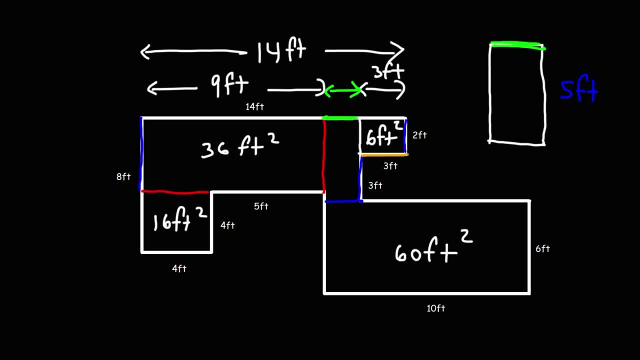 The sum of 9 and 3 is 12.. 14 minus 12 is 2.. So the length of this rectangle- It's 2 feet long. 5 times 2 is 10.. So we have an area of 10 square feet. 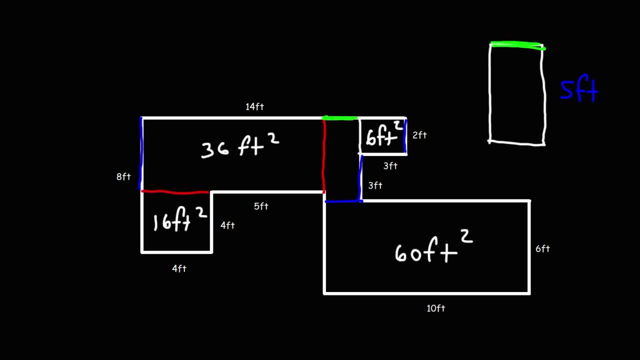 How can we do that? Well, we know this entire distance is 14 feet And if we add these two- 4 plus 5, we know that this section is 9 feet. And looking at this piece here, this is 3 feet long. 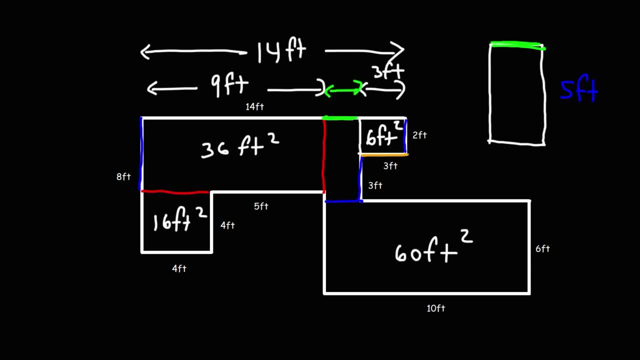 So to get the length of the rectangle, it's going to be the difference between 14 and the sum of these two, These two numbers, 9 and 3.. The sum of 9 and 3 is 12.. 14 minus 12 is 2.. 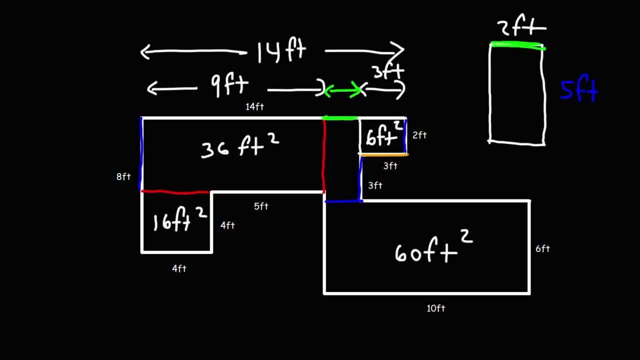 So the length of this rectangle- it's 2 feet long- 5 times 2 is 10.. So we have an area of 10 square feet. Now, in order to calculate the total area of the composite figure, we need to add up the area of the individual rectangles that we've created. 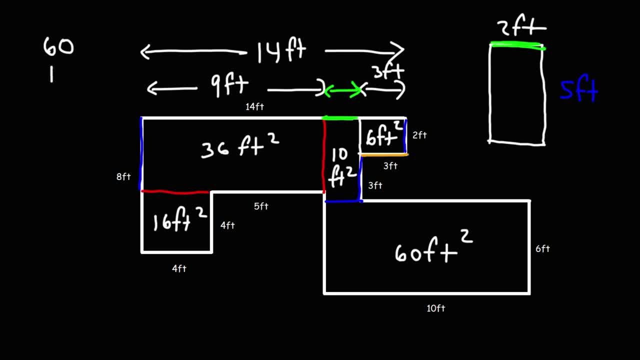 So let's start with. So we have 60 plus 10,, and then 36,, 16, and then the last one, which is 6.. So add in 6 three times, that's going to be 18.. 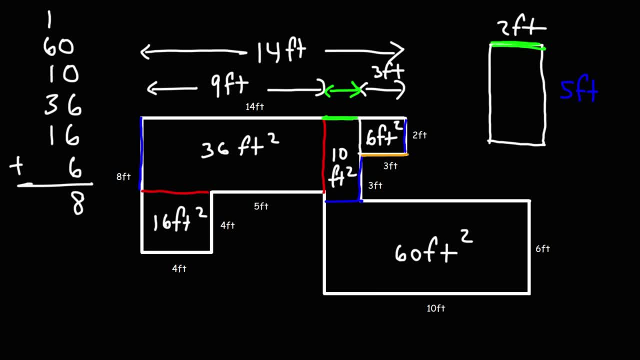 So we're going to write the 8, carry over the 1.. 1 plus 6 plus 1 is 8, plus 3,, that's 11, plus 1 is 12.. So the total area of this figure is 128 square feet. 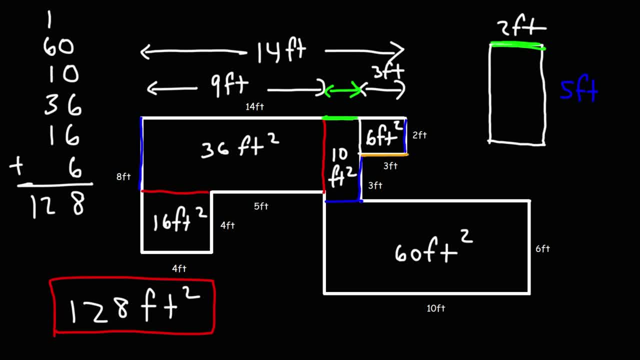 So that's how you can calculate the square feet. So that's how you can calculate the square footage of an area. You could use this, let's say, if you need to calculate the square footage of a floor plan, Let's say of your home or of an apartment. 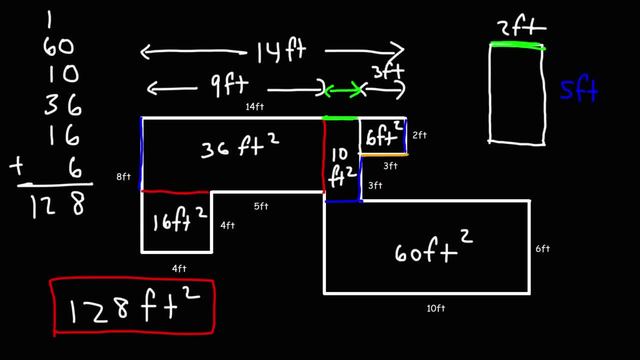 So this is some practical applications of understanding how to do this. That's it for this video, For those of you who like it. thanks again for watching And don't forget to subscribe to this channel. 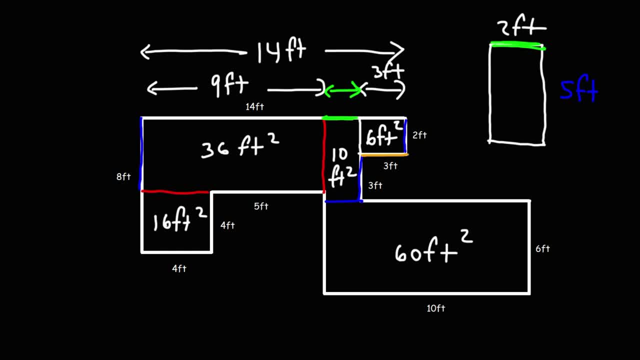 Now, in order to calculate the total area of the composite figure, We need to add up the area of the individual rectangles that we've created. So let's start with 60. Plus 10. And then 36., 16. And then the last one. 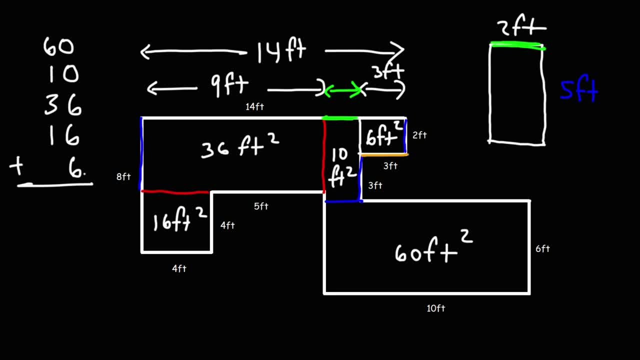 16. 6.. So add in 6 three times, that's going to be 18.. So we're going to write the 8, carry over the 1.. 1 plus 6 plus 1 is 8, plus 3, that's 11, plus 1 is 12.. So the total area of this figure is 128. 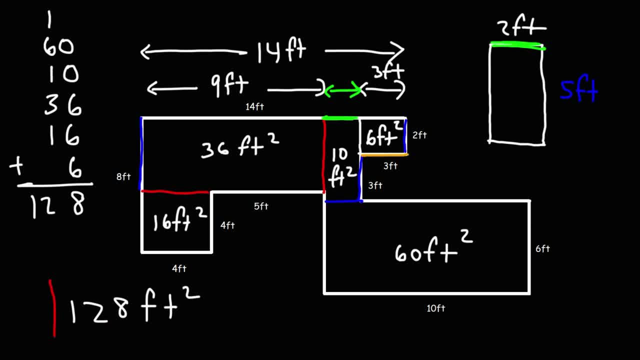 square feet. So that's how you can calculate the square footage of an area. You could use this if you need to calculate the square footage of a floor plan, let's say of your home or of an apartment. So this is some practical applications of understanding how to do this. Thus, that's it. 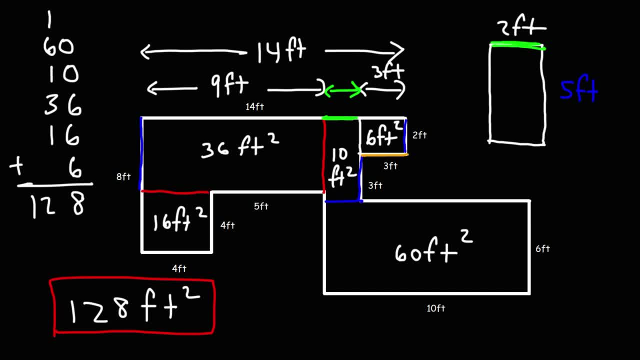 for this video For those of you who like it. thanks again for watching and don't forget to subscribe to this channel. 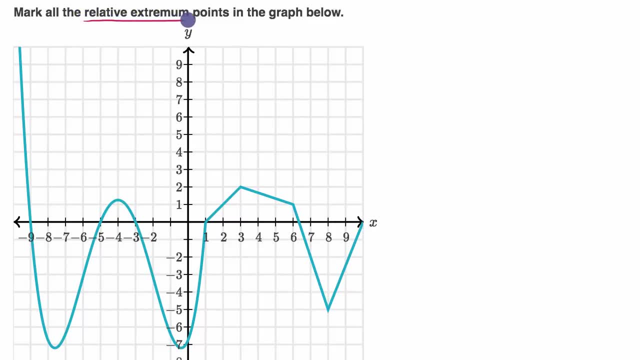 We're asked to mark all the relative extremum points in the graph below. So pause the video and see if you can have a go at that. Just try to maybe look at the screen and in your head see if you can identify the relative extrema.